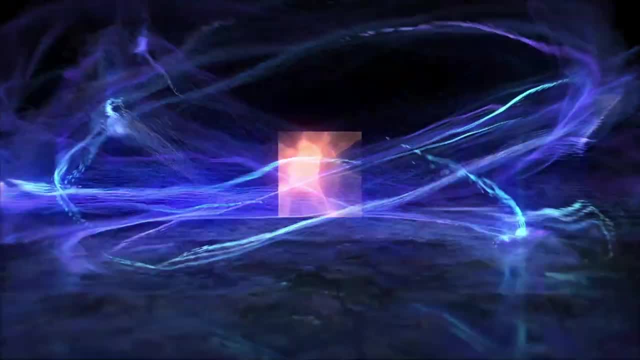 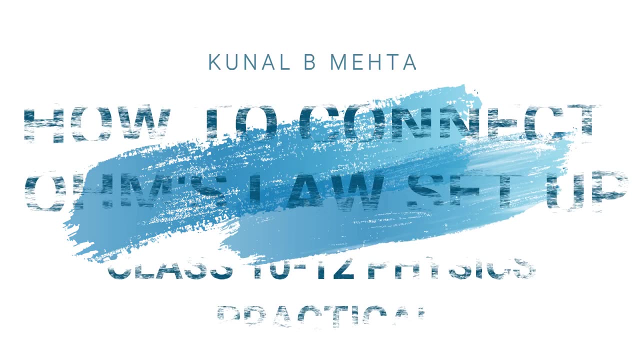 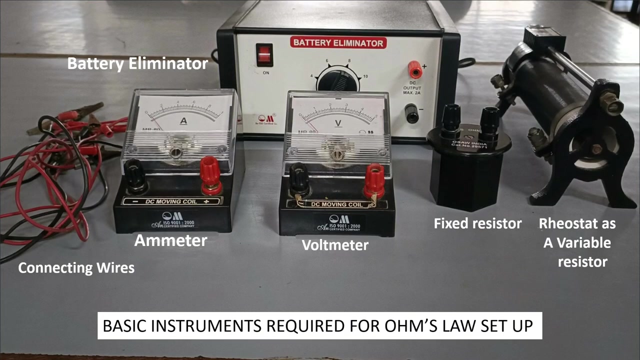 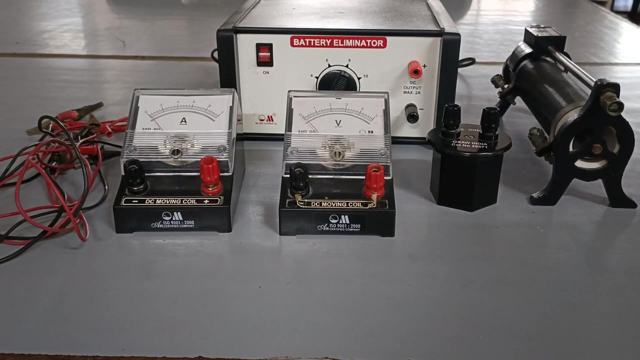 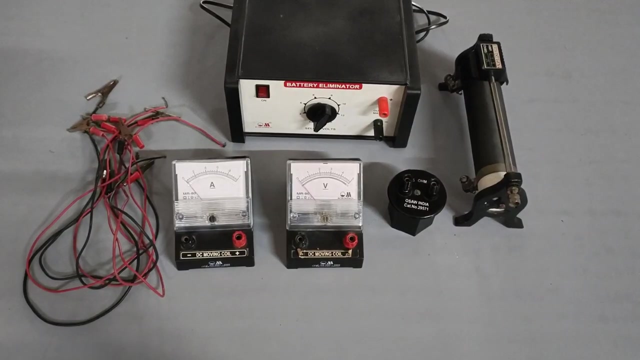 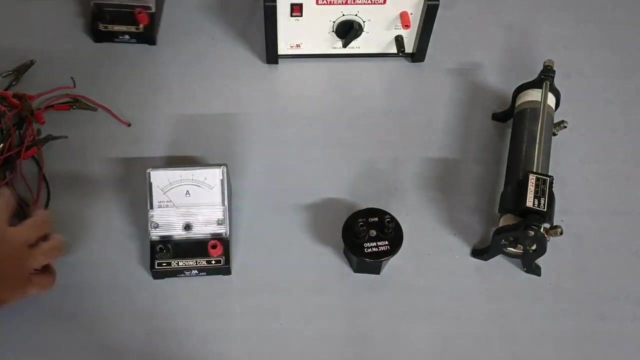 Hello everybody, welcome to our YouTube channel. Make Me Scientific. In this video I will show you how to connect the ohm's law circuit within 5 minutes. It's an electricity experiment as well as a standard 10 board practical. Let's quickly arrange the setup as shown. 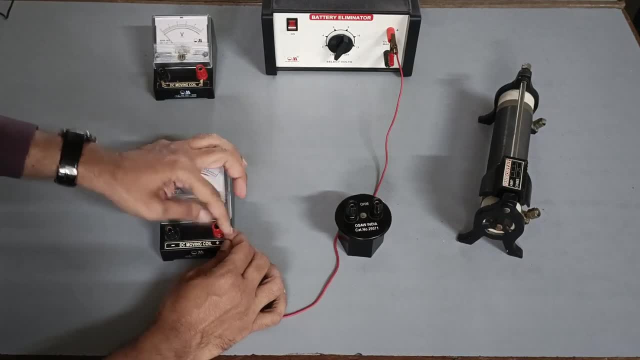 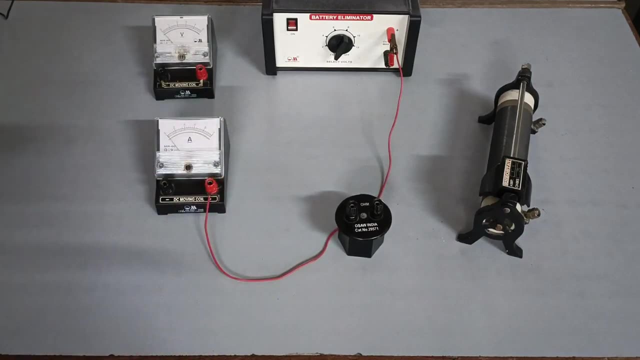 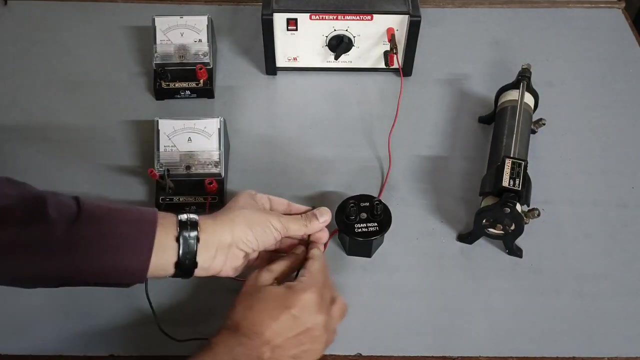 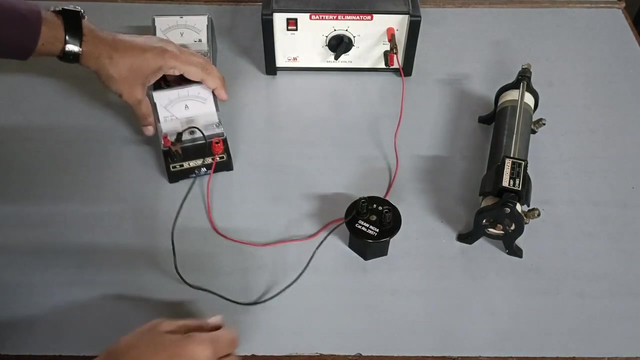 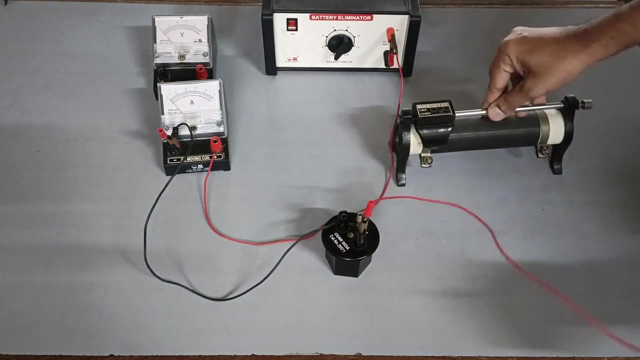 Let's begin: Connect the positive terminal of the battery with the positive terminal of the ammeter. Please note the red terminal is positive and the black one is a negative terminal. Please ensure the connections are tight. Negative terminal of the ammeter is to be connected to any one end of the unknown resistor whose value is fixed. The other end. 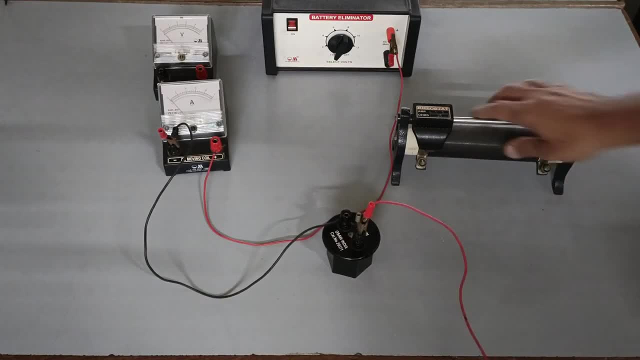 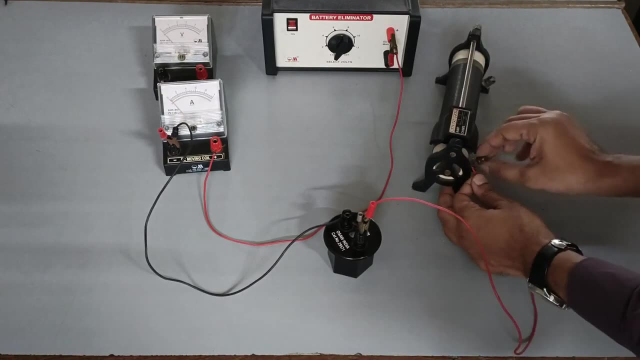 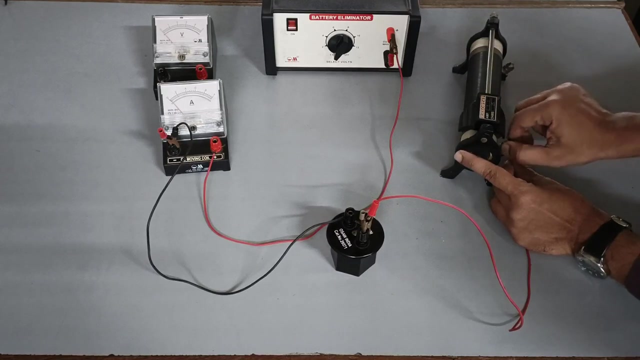 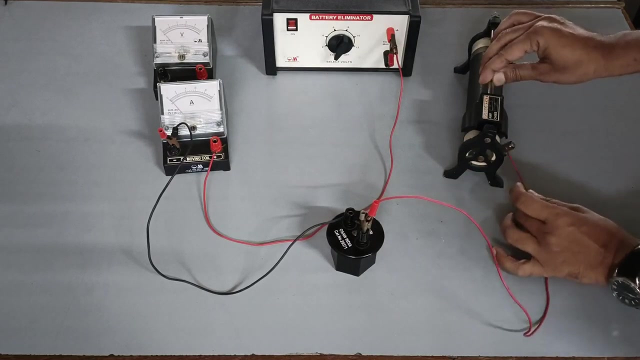 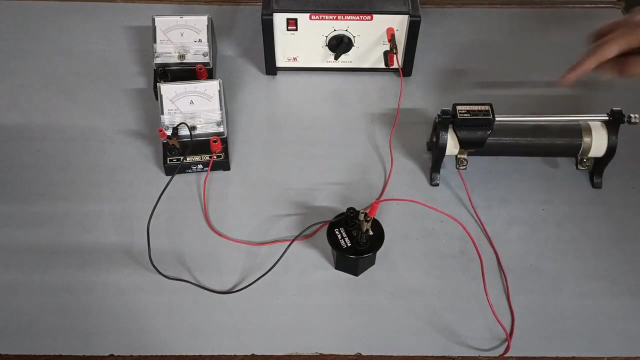 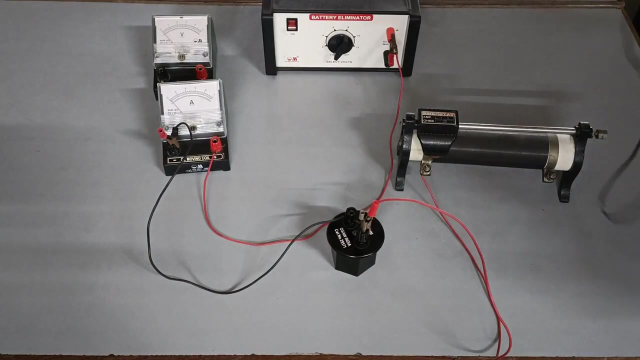 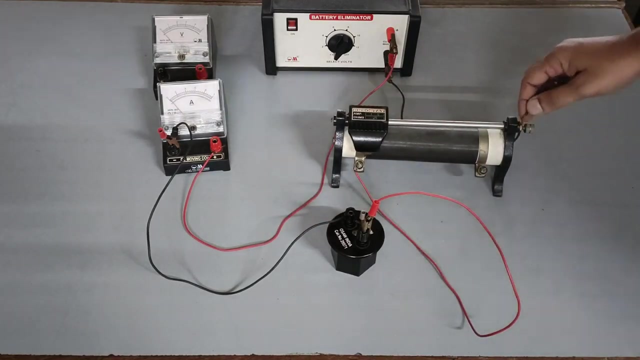 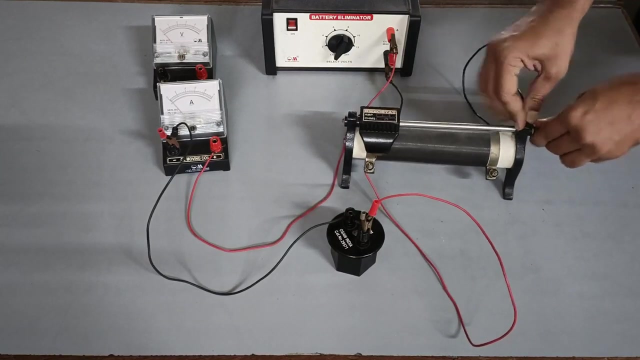 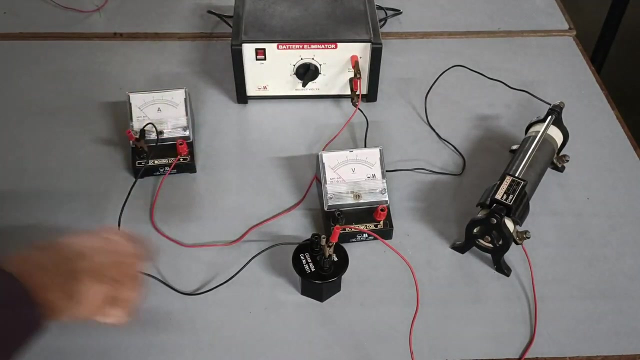 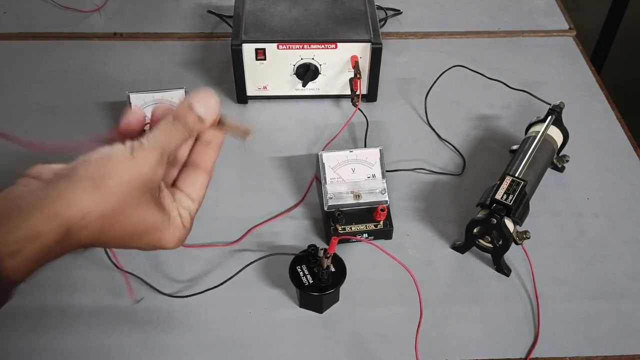 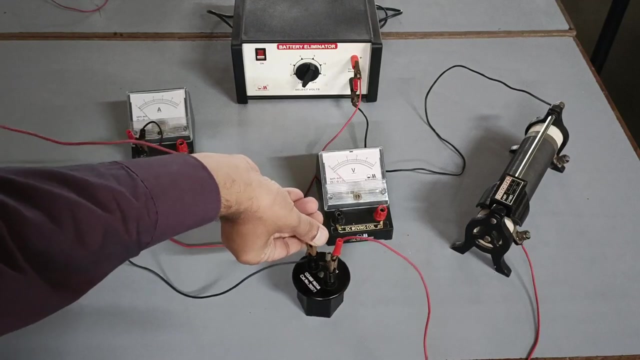 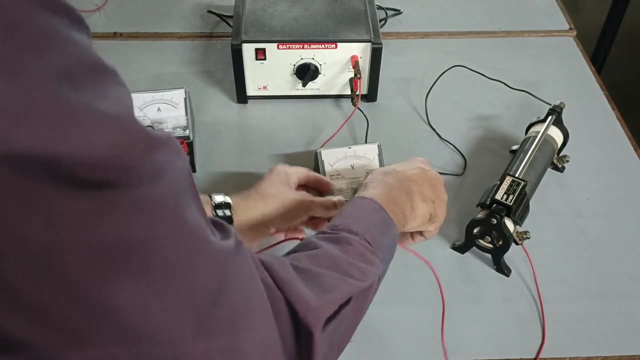 of the resistor is to be connected with these two terminals of the rheostat. The other terminal of the rheostat shall be connected to the negative terminal of the battery, The terminal of the resistor from which the current enters. the resistor has to be connected to the positive or the red one terminal of the voltmeter.